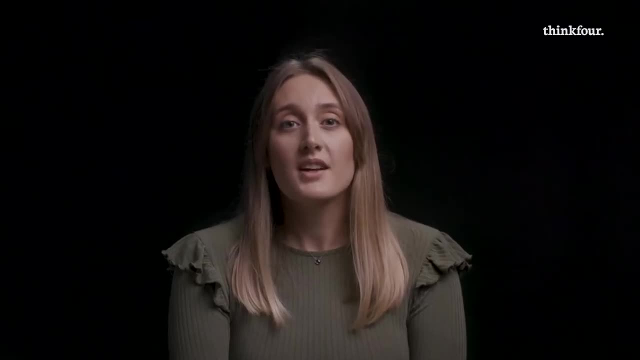 process of humification. Invertebrates such as worms are its engineers. They break down and mix the organic matter as they forage and feed, aerating the soil and aiding decomposition. Deciduous vegetation provides an abundant leaf litter that sustains the production of humus and its inhabitants, The deep roots. 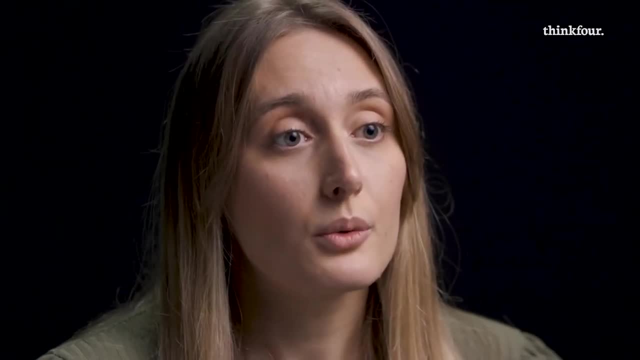 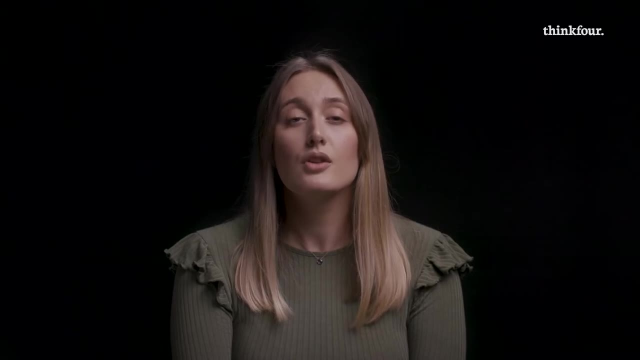 also recycle nutrients, promoting new plant growth and biota activity at the surface. This harmonious relationship is what soil scientists call the nutrient cycle. Our second soil forming process is leaching. It is a natural process by which water soluble minerals such as iron and aluminium are washed from the 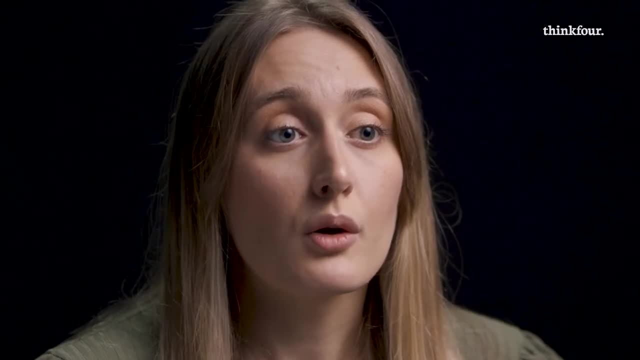 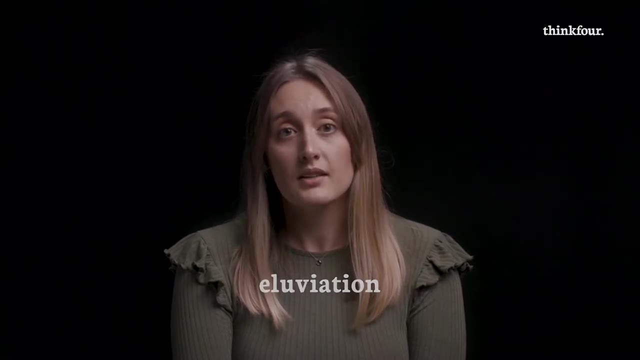 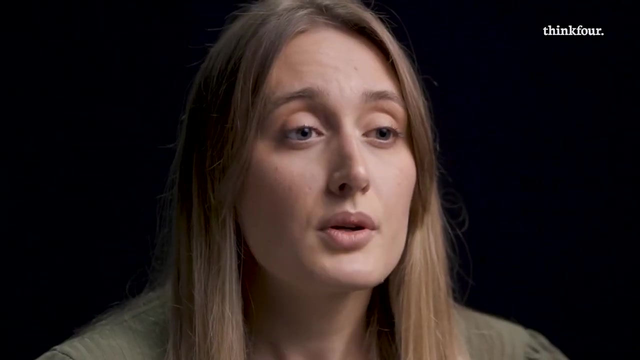 A horizon into the B. When minerals are washed from the A horizon, we call it eluviation. when they are washed into the B, we call it eluviation. Leaching is most associated with pod soils, as it promotes the formation of an iron pan When precipitation is greater than evapotranspiration. 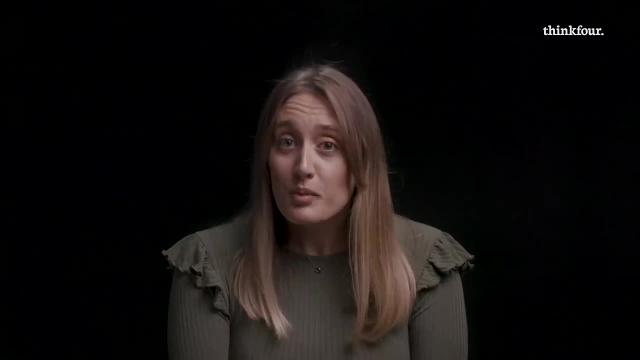 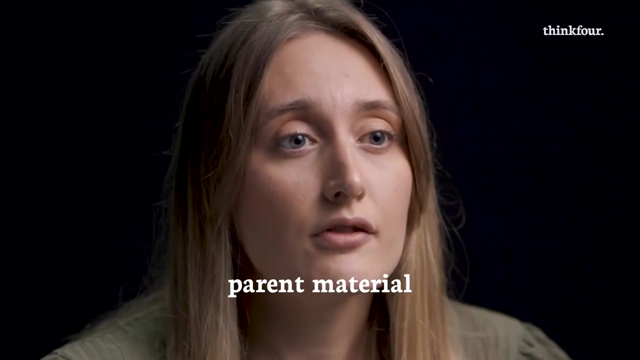 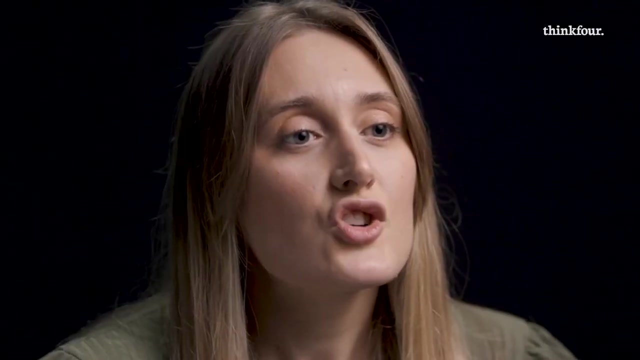 leaching intensifies, So it's no surprise to find that Scotland has its fair share of pod soils. The chemistry of parent material is a key factor influencing this process. Parent material is the bedrock that soil has formed on top of Soil is intrinsically linked to the characteristics of its parental base. 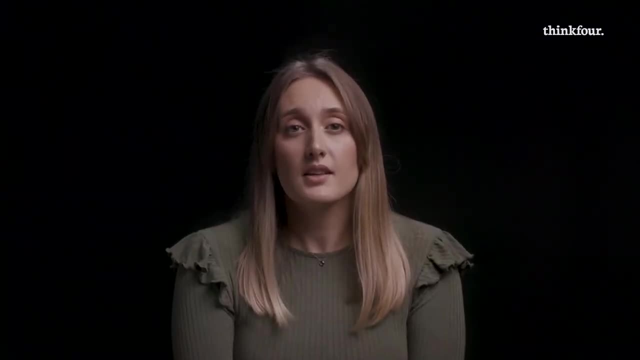 just like the genetics between children and their parents, Soil is intrinsically linked to the characteristics of its parental base, just like the genetics between children and their parents. A common rock lying beneath Scottish pod soils is granite, an acidic rock because of its mineral silica. But how does this influence the process of leaching? Well as 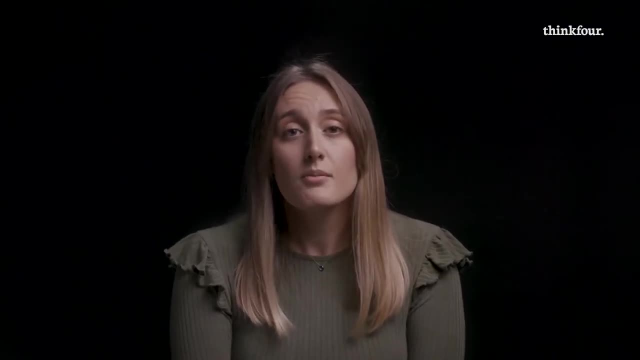 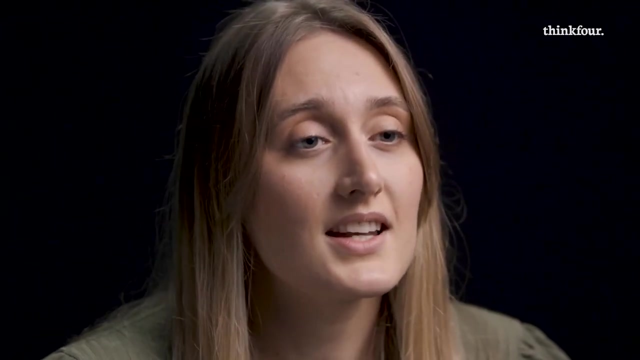 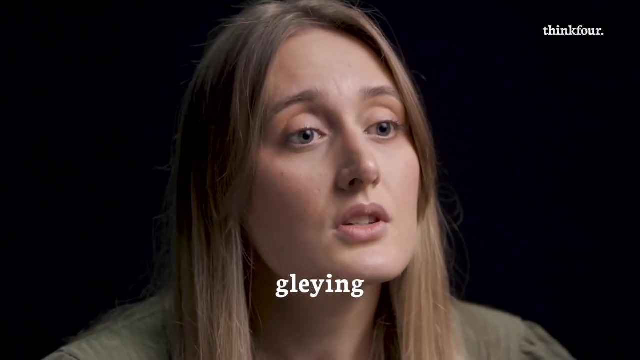 rainwater filters through an acidic soil, it too becomes acidic and breaks down iron and aluminium into more soluble particles, making them easier to eluviate. Therefore, without the acidity of its parent, rock, pod soils would not form their characteristic iron. Our third and final process is glaying the water logging and deoxygenation of soils. 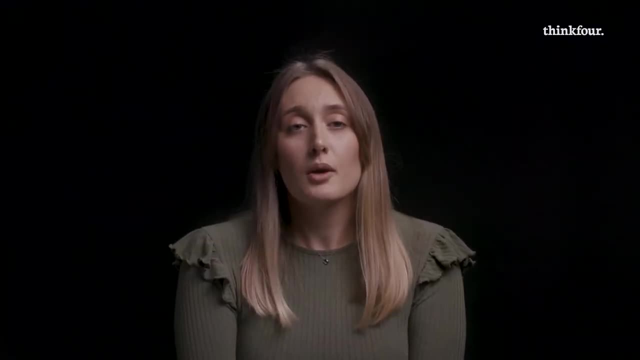 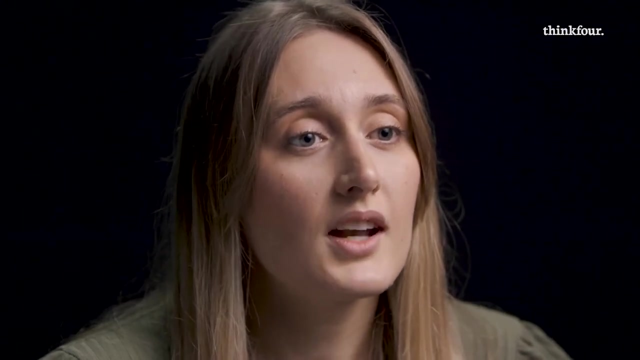 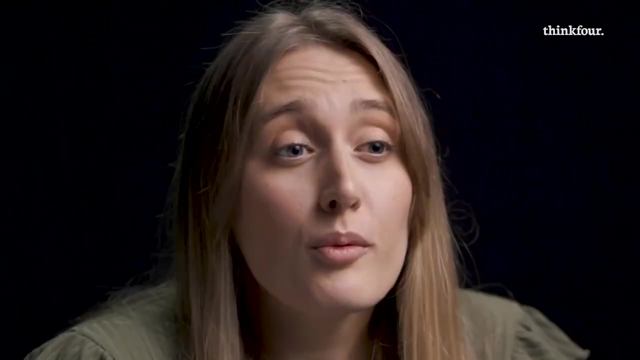 It is the process that gives glays their characteristic blue-grey horizons. Glays love the west coast of Scotland and blanket most of the outer Hebrides. I know I'm in a glay when I feel that slow ingress of water into my boots.